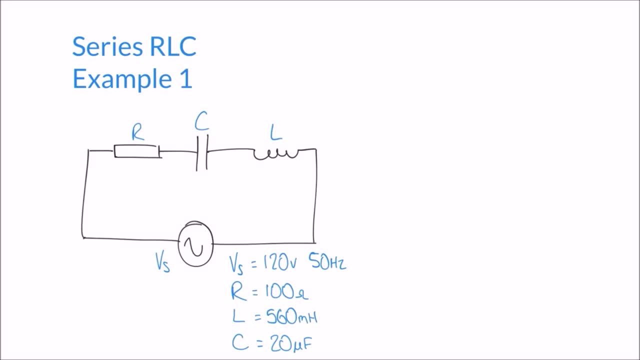 of components and the impedance of the whole circuit, And we're also going to calculate currents and voltages within the circuit. It is worth mentioning that in this example we're going to be doing calculations and answers in polar form or in complex numbers. If you're not so sure about complex numbers, it's worth going back and checking out the 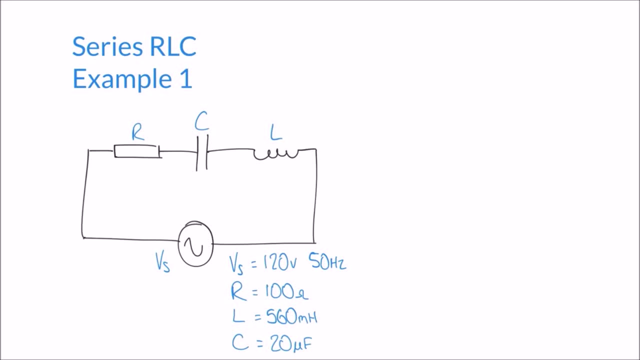 videos on that topic. But let's first of all begin by defining the reactance in this circuit. We have three components here: resistance, capacitance and inductance in the circuit, And inductors have the property of reactance when they're in an AC circuit. So let's begin. 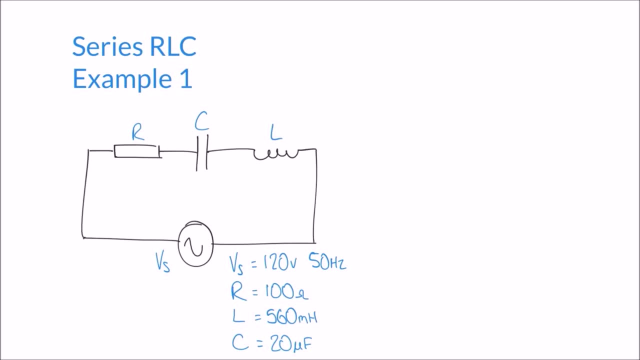 first of all by calculating the reactance of our inductor L, And we'll call that XL the reactance of the inductor. And we know that the formula to calculate the reactance of an inductor is 2 pi FL, 2 pi times the frequency times the inductance. So substituting 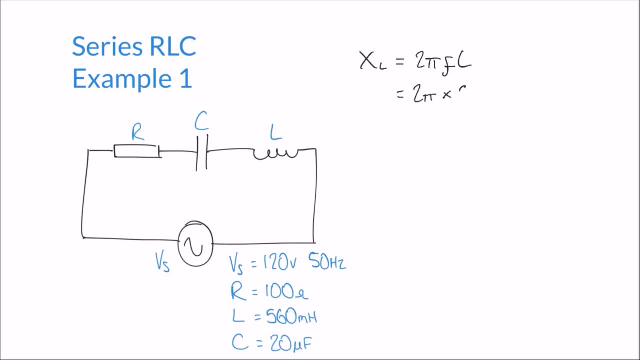 some values in here: 2 pi times the frequency, Which is 50, 50 hertz Times by L, the inductance, which we said is 560 millihenries. So that's 560 times 10 to the minus 3.. And calculating that gives me an answer of 175.93 ohms. Let's 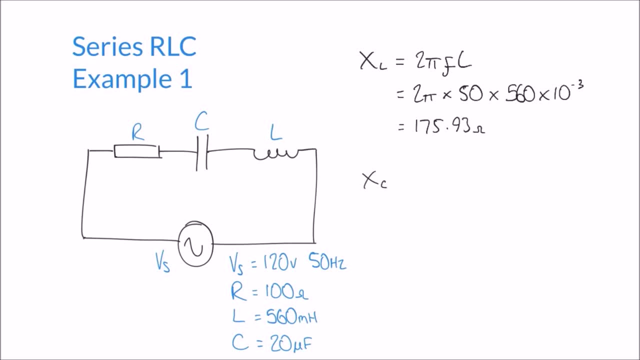 do something similar for the reactance of the capacitor, the other reactance in our circuit, XC, And the formula for the reactance of the capacitor is 1 over 2 pi FC, And likewise we can put some values in here. We can see that that is 1 over 2 pi times 50, the frequency Times. 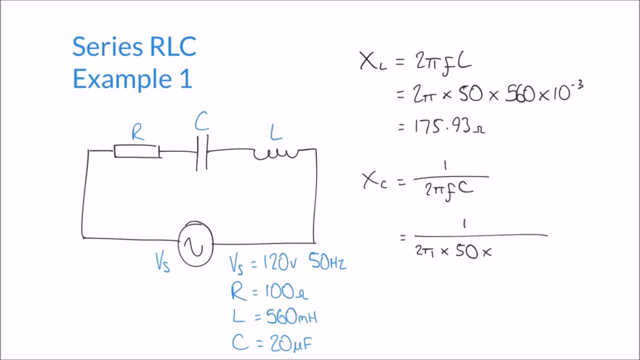 C, which is our capacitance, which in our case is 20 microfarads, 20 times 10 to the minus 6.. And that comes out with an answer of 159.15 ohms. The next step in this particular circuit is: 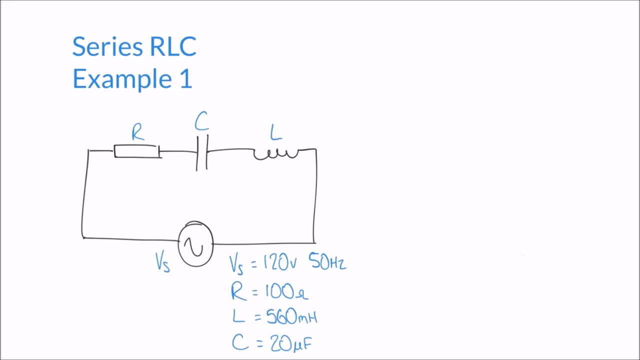 to calculate the impedance of the whole circuit. And the impedance is really the combination of both the resistance and reactance in the circuit. Now the 10 times the impedance of the whole circuit is the resistance. so the impedance gives us negative one cast radius. This Party M by Denyang's filter will grab Luca. Let's do this And we don't need to do that now. This is the resistance of larvae. Now, the only property we can use for the Dahax- We've done this in this circuit- is- is to now take the fat in the amount of authentic solidizedjing. 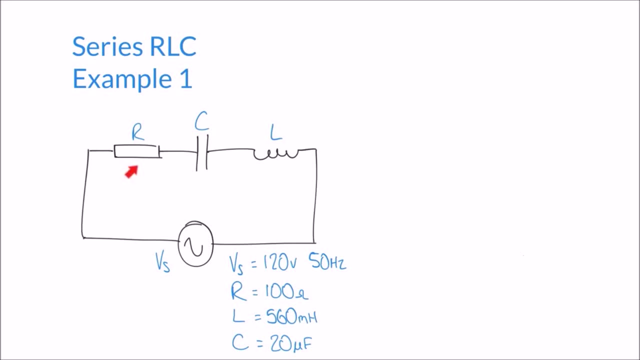 temptation is to say: well, because resistance is measured in ohms and the reactance is that we've both calculated are both measured in ohms. the impedance is simply just a case of adding all three of these parameters together. now, unfortunately, it's not quite as simple as that, and I'll try to illustrate with. 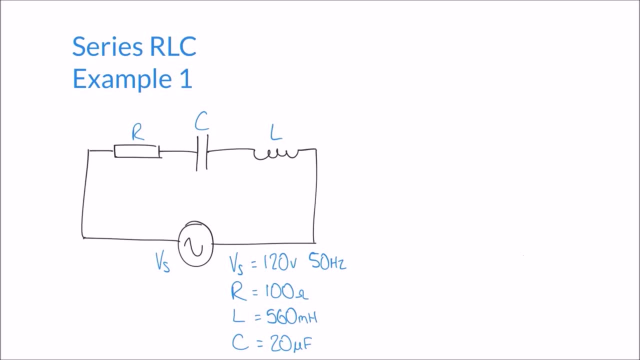 us with a sketch. we're going to try and represent our resistance and our reactance as a complex number, and to do that we need two sets of axes. so resistance is going to be a horizontal axis going along the bottom here and reactance is going to be a vertical axis going up the side. and this is because 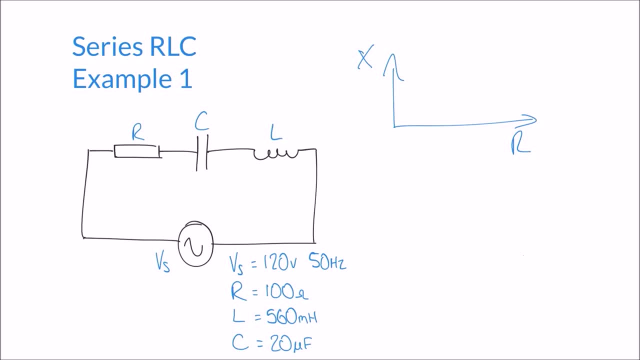 we're representing resistance as a real number going along our sort of x-axis, as it were, and reactance is what's called an imaginary number going up the y-axis, and together we're going to use those to calculate our impedance. now we have two reactance in this circuit. we have the. 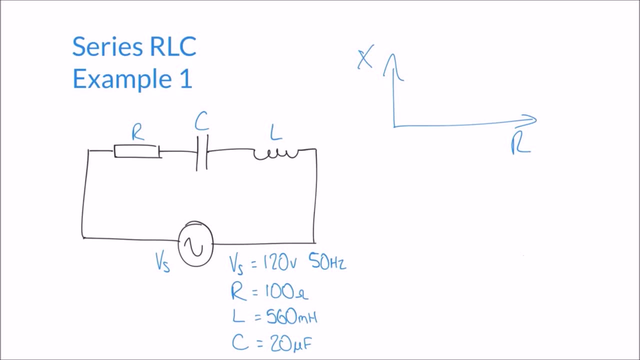 reactance of the inductor and the reactance of the capacitor and as such, we have to represent both on our diagram and the way we do. that is actually by representing the reactance of the inductor, the inductive reactance as a positive number going up, and the capacitive. 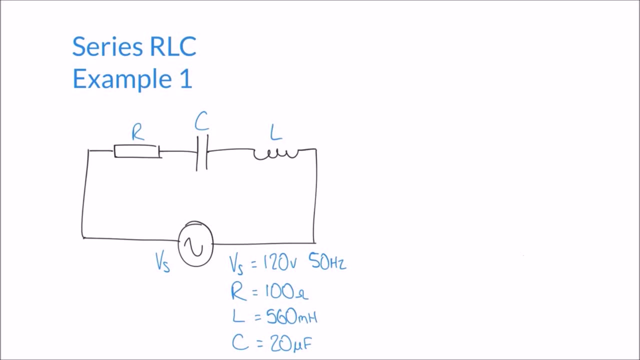 reactance as a negative number going down. but they're both on the sort of y-axis, the imaginary scale, in our complex number. again, if you're not sure about complex numbers, it's probably worth revisiting the topic before tackling the rest of this question. but let's plow on ahead and try and 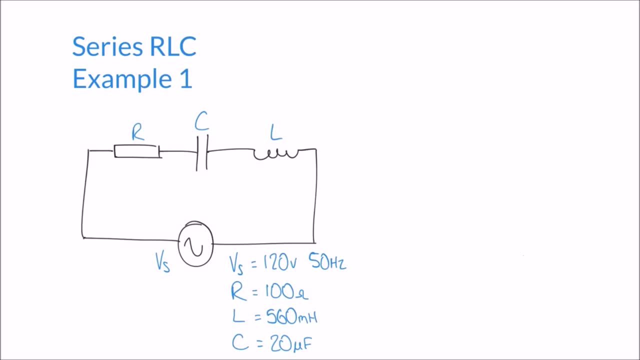 sketch this diagram. first of all, we have our resistance, which is going along here, and r is in our case 100 ohms, so i'll put that on my diagram as well. we've also calculated our inductive reactance, which was 175.93 ohms, so i'll pen that on here. xl is: 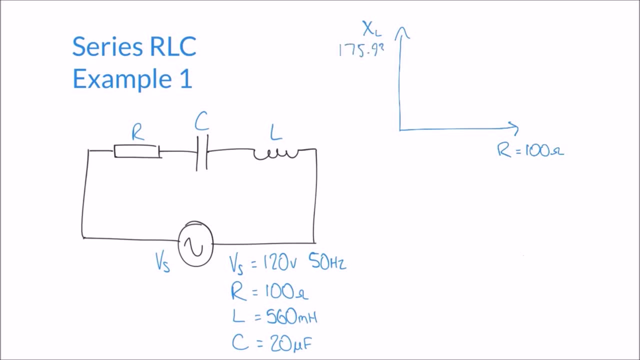 175.93 ohms, but we also have our capacitive reactants, and our capacitive reactants should always be in the downward direction, and that comes to a value of 159.15 ohms. that's what we calculated on the previous slide there. 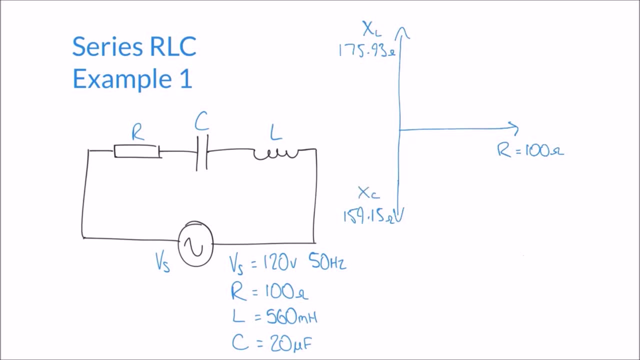 and that was XC. now, to simplify the process here, you'll see that we have our inductive reactants pointing in this upward direction and we have our capacitive reactants pointing in this downward direction. they oppose one another, and so what we can do is we can actually cancel these two down. 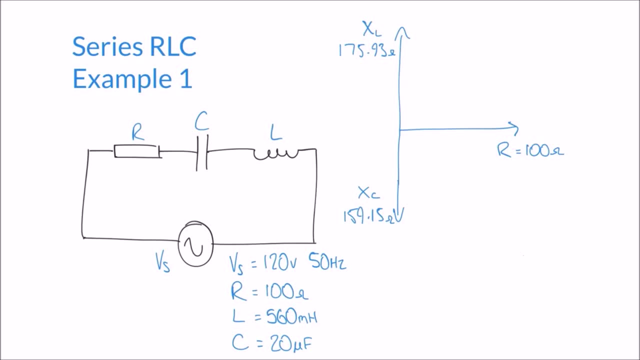 to simplify our diagram: if we have 175.93 going up and we have 159.15 going down, then we can simply calculate the difference between them, and the difference in this case works out to be 16.78, so 175.93 minus 159.15. 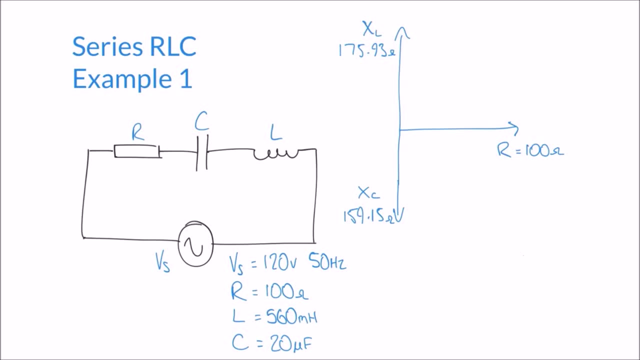 so we can simplify our diagram a little bit by doing away with both of these. so I'll take those out there and replacing it with just one simplified version, as it were, which is 159.15. the total reactants is going to look like this. it's going to be: 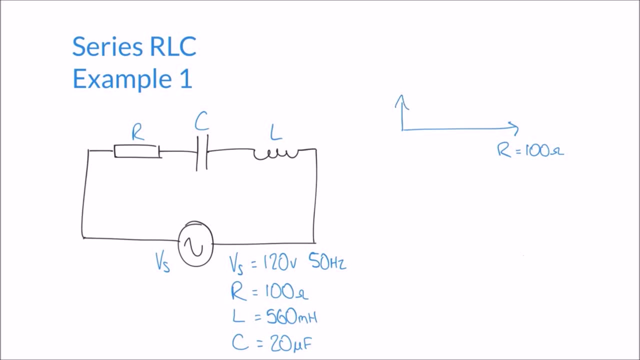 just whatever. the difference between them was 16.78 ohms, and I'm going to call that XT the total reactants. so that's taking into account both the inductive reactants going up and the capacitive reactants going down. so now that we've calculated, 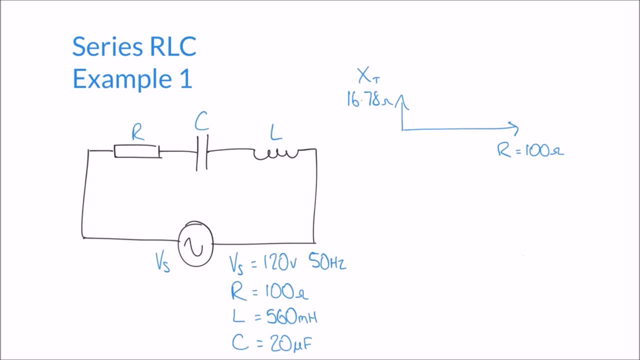 the total reactants in our circuit and we have XT and we're also aware of the resistance in our circuit. we can use both of these to calculate our impedance, And the best way to do this is to visualize our impedance triangle. So if we have our resistance going off to the side and our reactance going up the side there, 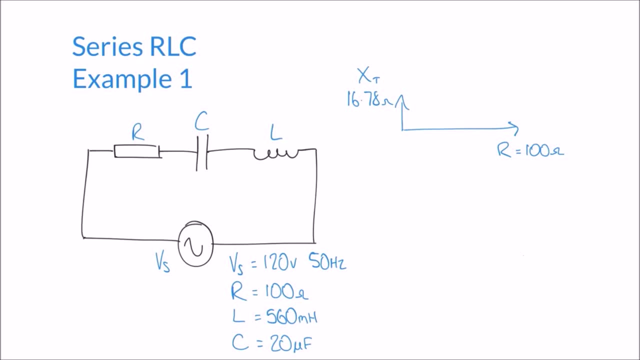 then the resultant of these two is going to be our impedance, And I'll try and draw that on like so. So our impedance, if you can imagine, being the sort of completing the hypotenuse of this triangle that we have here, where the side, the vertical side, is 16.78 and the horizontal side is 100. 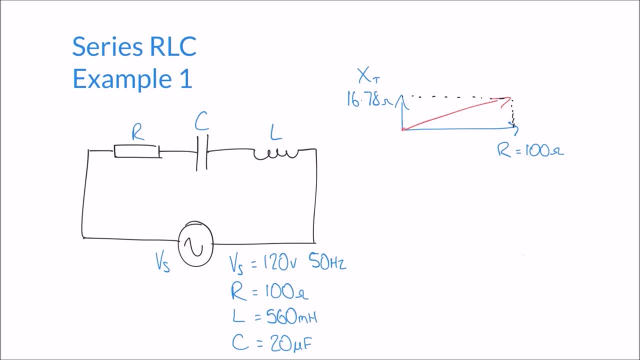 So, to calculate the length of our sort of diagonal, our hypotenuse there is actually going to give us the impedance of our circuit And, as a result, we can use, We can use Pythagoras' theorem, We can say that Z squared, the hypotenuse, as it were. 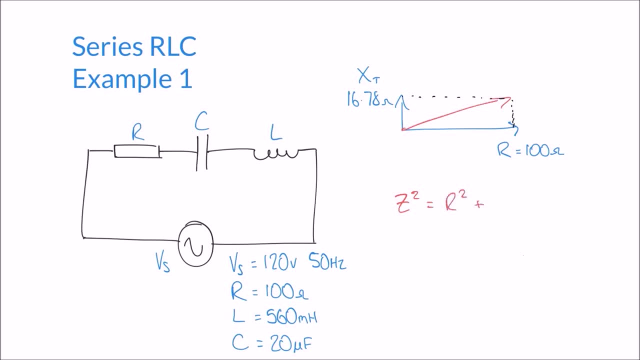 is equal to R squared plus XT, the total reactance squared, And so substituting some values in here, R is 100, 100 ohms, so 100 squared plus, our total reactance squared, we said, was 16.78 squared. 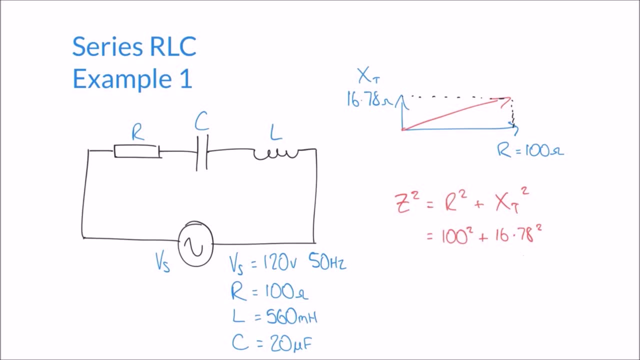 And calculating, And that gives me a very large number: 10,281.57.. I'm not too interested in that number because I'm not calculating Z squared, I'm just calculating Z And so I want to find the square root of that number. 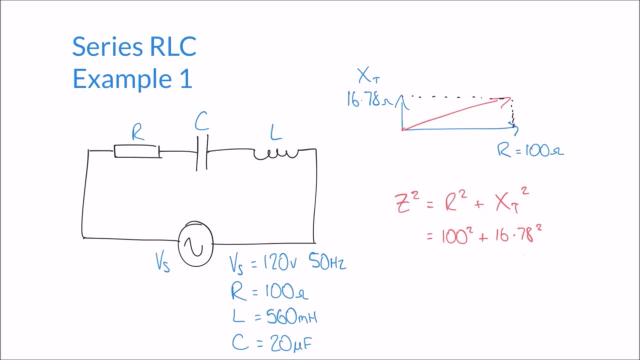 Z squared is 10,281.57.. But Z is only going to be the square root of that, which is 101.40.. Now add this up to I over 0.. I give it to him. I give it to him. 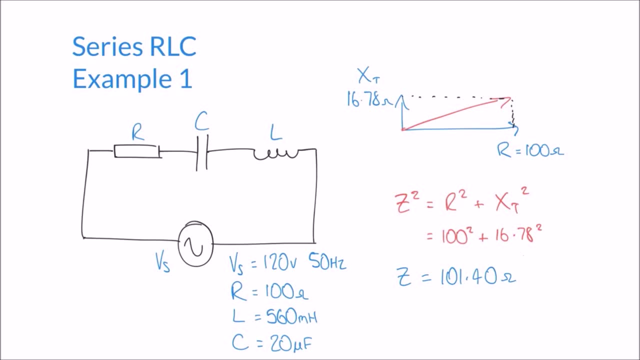 And we get that value at one point and we're gonna put my Als And when your к. So that's what I can call an angle. now, Okay, really easily, using trigonometry as well, if we know our trigonometric identities, we can say: 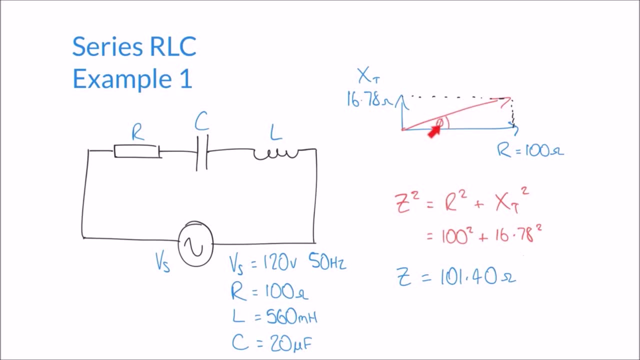 that here's our hypotenuse and here's our marked angle. so this side of the triangle, as it were, which is the same length as this side, this side here is the opposite of the triangle and this side is the adjacent of the triangle and so one of the one of the best identities to use in this. 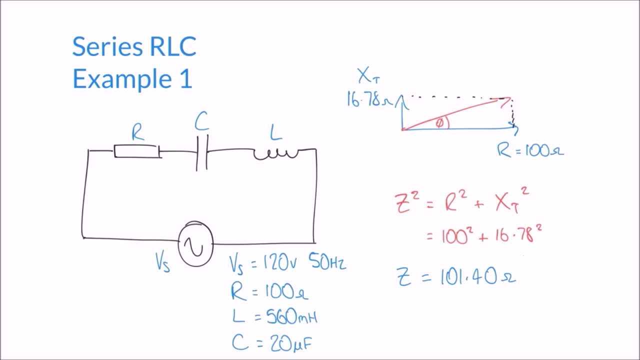 case would be the tan identity tan of the angle being equal to the opposite divided by the adjacent. we're going to rearrange that very slightly. we're going to say that the angle itself is equal to tan, to the minus one opposite over adjacent, and in our case the opposite is 16.78. 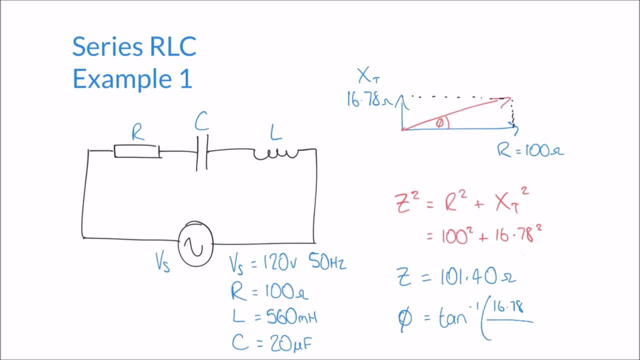 and the adjacent is our resistance 100, and if i calculate that and if i calculate that, i get an angle of 9.53 degrees. so now that we've calculated the impedance of our circuit, we can go ahead and calculate the current that flows through our circuit. we have a series circuit, so there's only one current, the same. 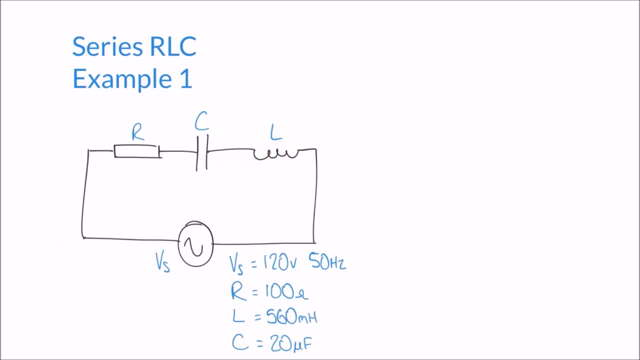 current flows through all three of our components and we can calculate that by using ohm's law. so we're going to calculate the impedance of our circuit by using ohm's law. so we're simply going to say that the current i is equal to v over z, the voltage divided by the impedance. 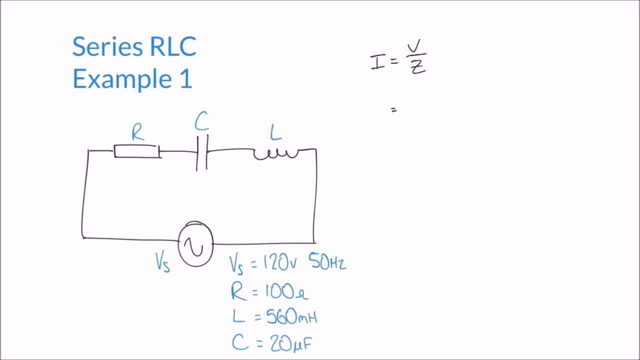 so in this case we're going to continue to use polar form in our calculation. so the voltage is 120 volts, But we're going to say that that's 120 volts at an angle of 0 degrees. In this case, our supply voltage is our reference phasor, and so that's going to be at 0 degrees. 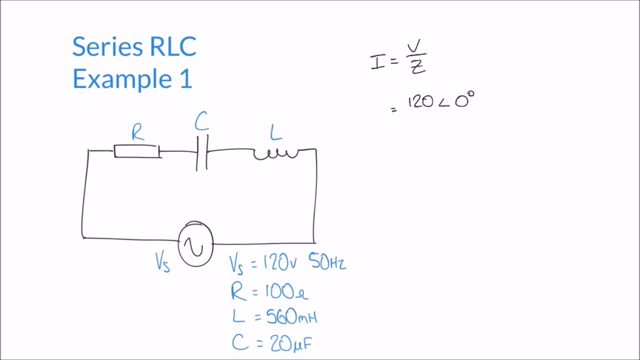 And we know from our previous slide that the impedance comes out at a value of 101.4 at an angle of 9.53 degrees. And so when we're dividing in polar form, we divide the actual first term, the number of the answer, and we subtract the angles. 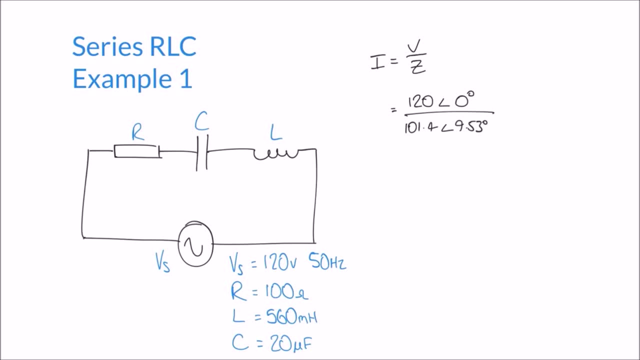 So we'll end up with a result of 1.18 at an angle of minus 9.53 degrees. Now that we have the current that flows through the whole circuit, the last thing that we can calculate in this circuit is the voltage across each component. 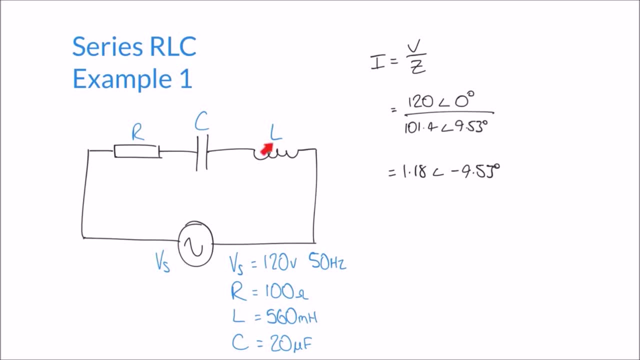 We know the supply voltage, the voltage that's supplied to the whole circuit. but some of that voltage will be dropped across the resistor, some of that voltage across the capacitor and some of that voltage across the inductor. So what we can do is again use Ohm's law. 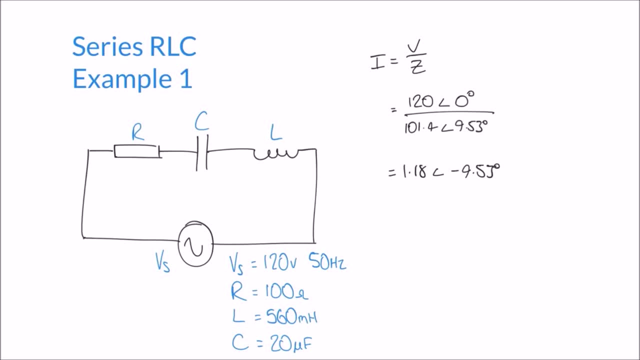 To work. in this case, we're going to use Ohm's law And we're going to work out the individual voltages dropped across each component. Let's begin by calculating Vr, the voltage across the resistor, And so Vr, again using Ohm's law, is going to be current I multiplied by the resistance R. 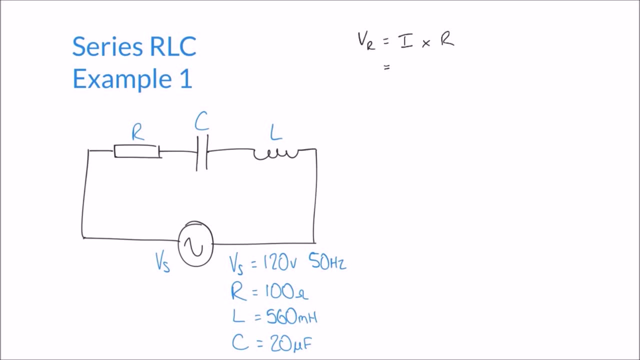 We know the current I from our previous slide. We said that it was 1.18.. At an angle of minus 9.53 degrees And we're multiplying it by the resistance- The resistance we're given in the question, 100 Ohms. 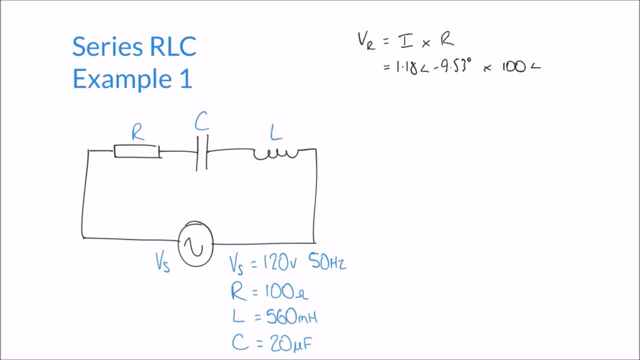 And again we're trying to use polar form. Resistances don't have a phase angle, So it's 0 degrees. Multiplying those two terms, We can say that we have an answer of 1.18 multiplied by 100, at an angle of minus 9.53 plus 0.. 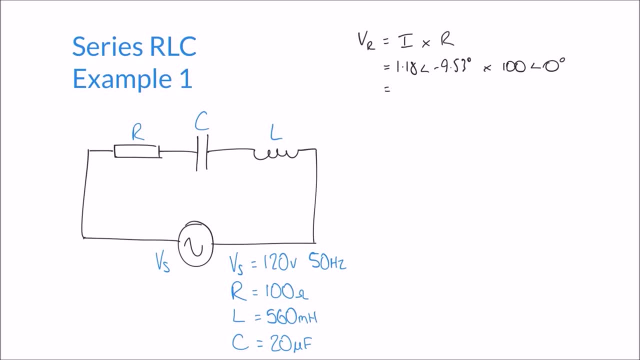 We multiply the numbers themselves and we add the angles when we're multiplying in polar form, And so we get a result of 118 at an angle of again minus 9.53.. And that's a voltage, so volts. Let's do exactly the same for the capacitor in our circuit. 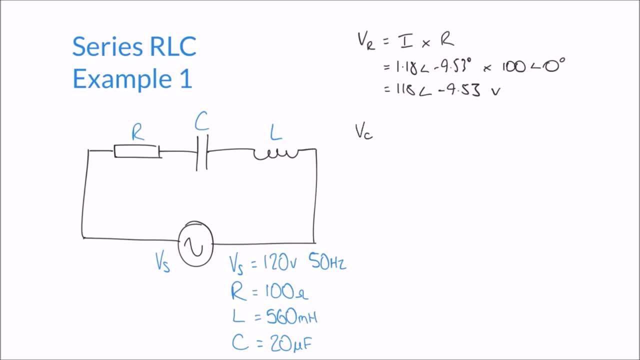 So Vc, the voltage across the capacitor, is again going to be I, the current multiplied by, not the resistance this time, but reactance Xc, the reactance of the capacitor, And so we can substitute R Values in. once again we can say: the current is the same, current 1.18, at an angle of minus 9.53. 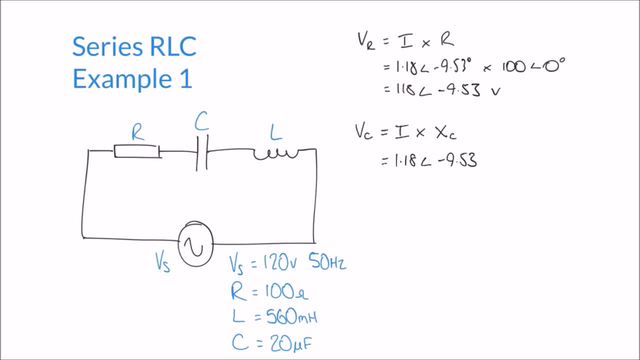 We can also say that our reactance, which we calculated right back at the start, is 159.. We can also say that our reactance, which we calculated right back at the start, is 159.15.. And, remembering that it's a reactance and not a resistance, we'll have to include a 90 degree phase shift. 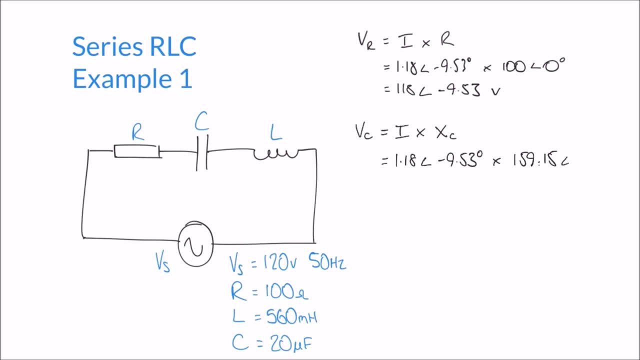 So capacitors. their reactance is at minus 90 degrees relative to a resistance. So again, multiplying those two terms, we come out with a result of 187.8.. At an angle of minus 99.53 degrees, And again that's a voltage. 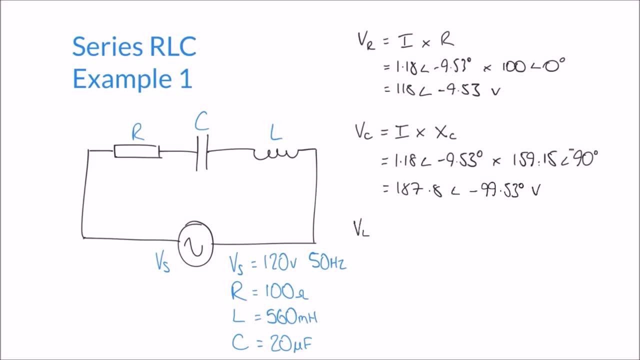 Lastly, exactly the same method. once again, VL is going to be. I times XL And the same thing applies. Our current is 1.18.. At an angle of minus 9.53.. Multiplied by the reactance of our inductor. 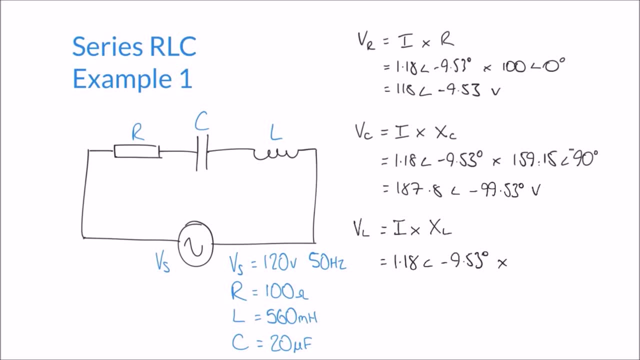 And, just like capacitors, inductors also have a reactance. The reactance also has a 90 degree phase shift, But this time their reactance is at 90 degrees relative to a resistance. Our reactance, if you remember, was 170.. 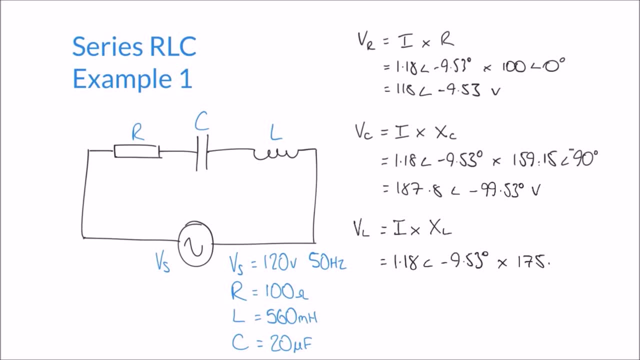 We now have 275.93.. And that will be at an angle of 90 degrees his time. So our final calculation is going to give us a result of 207.60 Multiplied at an angle of 80.47 degrees. The moment tensile area, where we mentioned key degrees, has a negative. 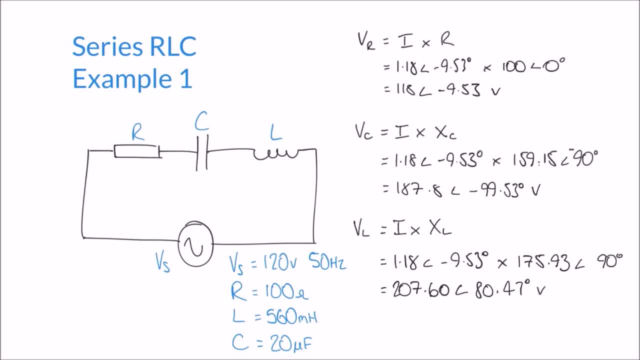 allowed. So the relationship is that degrees and again, that's our final voltage. So what we can see here is that we end up with three separate voltages across the three separate components. One thing you might notice is the size of these voltages actually comes to a total far greater than our original supply voltage. 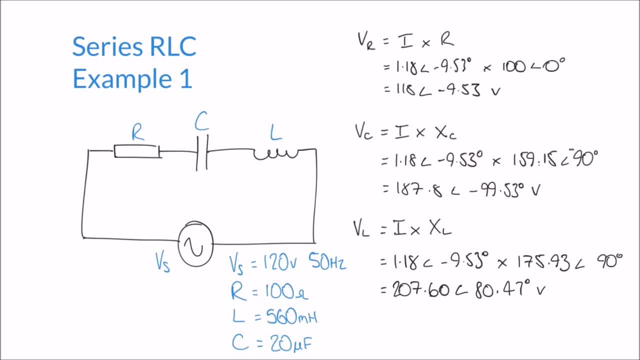 and there's a reason for that. it's called voltage magnification, and it's one of the strange effects of our series circuit, The reason being we also need to take into account the direction of our phasors, and so what we'll find is that 187.8 volts is actually pointing in a fairly 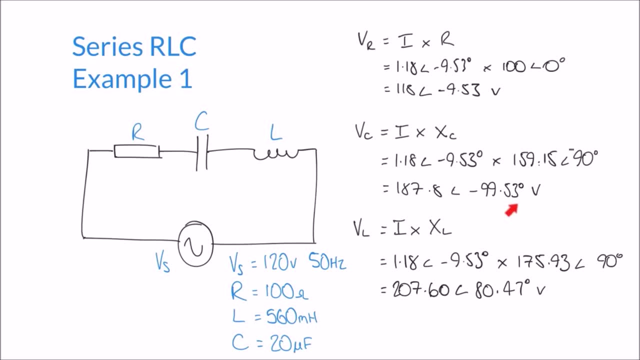 downward direction with this negative phase angle. but our 207.6 volt voltage is actually pointing in a fairly downward direction with this negative phase angle. but our 207.6 volt voltage is pointed upwards or tilted upwards with its phase angle being positive, and so these two in total will somewhat cancel out and will leave us with a total of what we originally 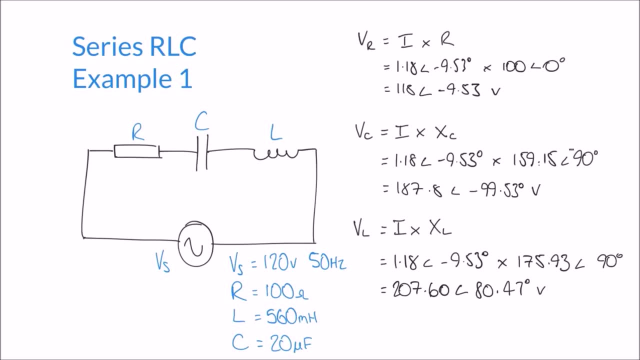 set out with our supply voltage, but when measured individually we can actually get some very high voltages. so voltage magnification is one of the unusual features of series RLC circuits. So I hope you found this video useful, first of all on looking at series RLC circuits and being able 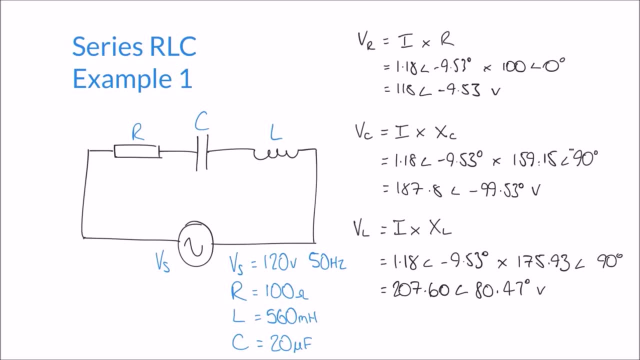 to calculate the currents and voltages within them. We're going to look at some more examples in later videos of RLC circuits and also the concept of resonance.